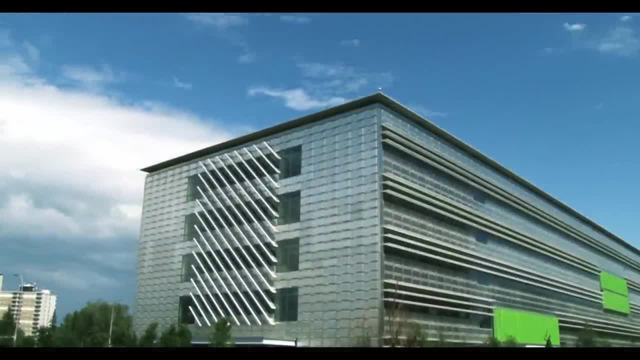 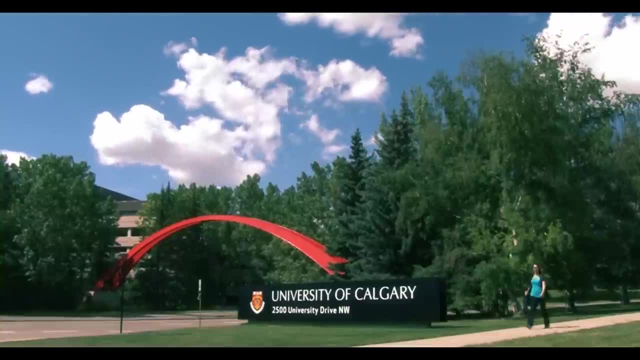 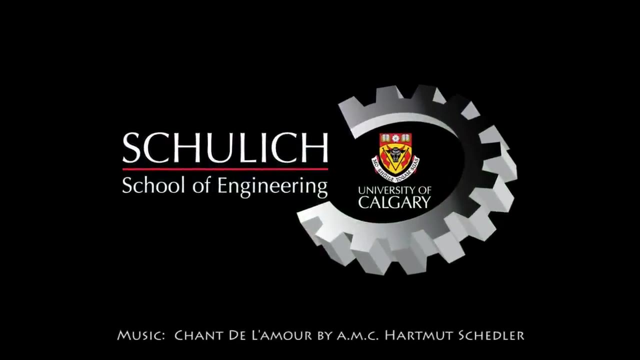 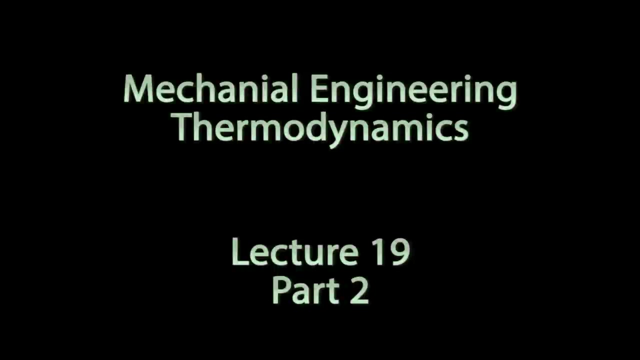 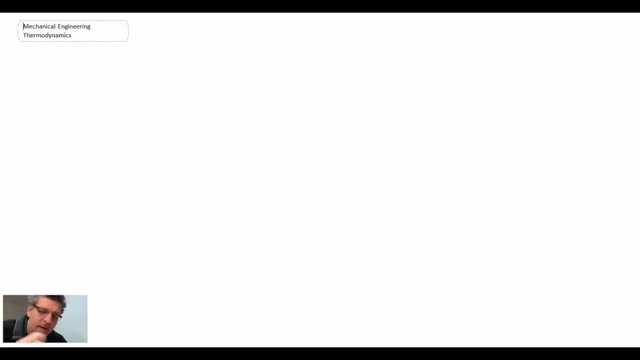 Now the most popular, well-known vapor powers cycle is referred to as being the Rankine cycle, And so that's what we'll start with, And we'll be looking at the conventional Rankine and then derivatives or modifications to that. So what I'll do to begin is I'll write out the process schematic as well as the process diagram. 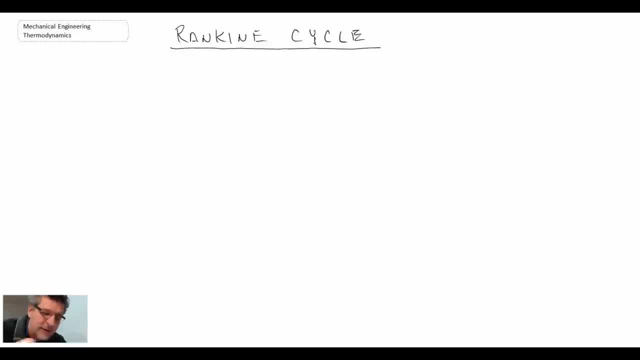 for the Rankine, and then we'll go through and apply the first law to each of the individual components in this cycle. So what we have with the Rankine cycle- you can see the schematic on the left- and we have a pump. 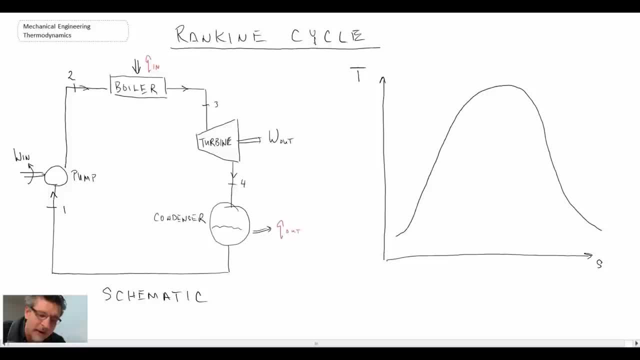 The fluid comes out of the pump, goes into a boiler where we have heat addition. It converts into steam. The steam then goes into a turbine, produces work, The steam comes out of the turbine and we condense it back into a liquid phase and then bring it back into the pump. So what we're going to do? 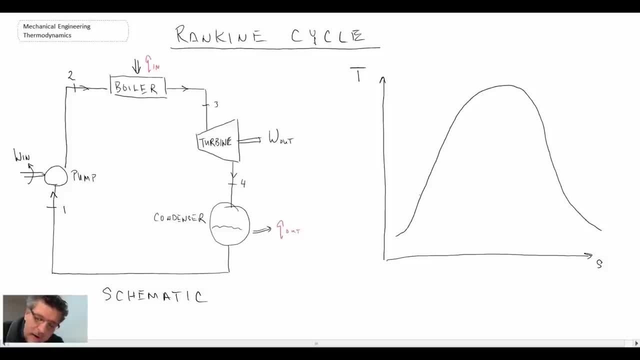 now is. let's represent that in the diagram, the process diagram, in the TS. So we always start off on the saturated liquid line and that will be state one, which is where we then go into the pump. And when we go through the pump, what we're doing is we're raising the pressure of the fluid. 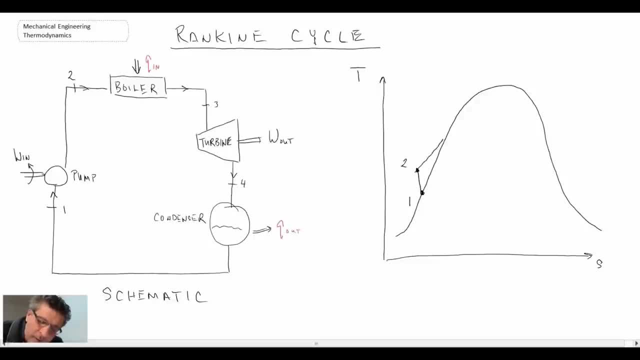 taking us to state. And then we have a constant pressure line, because we will assume that the operation in the boiler is a constant pressure. We'll see later that that's a bit of an approximation, but it's one that we'll use for now. 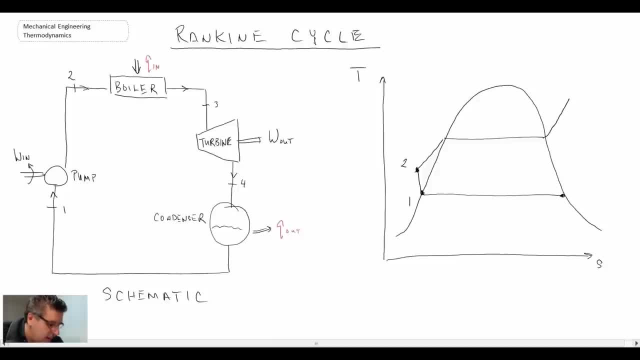 And then, once we go through the pump- so we're doing work in here, so we'll represent that- We then go into the boiler taking us from state two up to state three, which brings us into the superheated region, And in order to do, 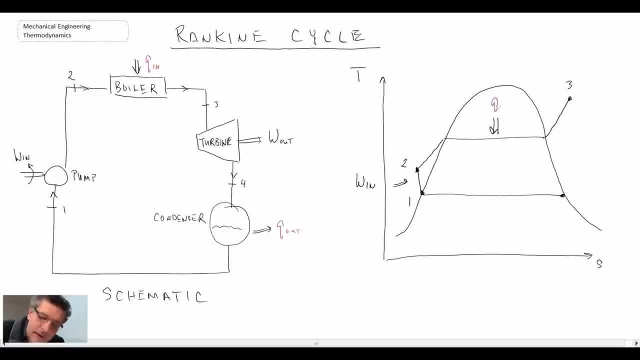 that we need to have heat addition. So that is what is going on in the boiler. We are then a superheated steam and we go into the turbine and we then drop down through the turbine. So we're dropping in pressure And ideally what will happen is we will end right on the saturated vapor line. 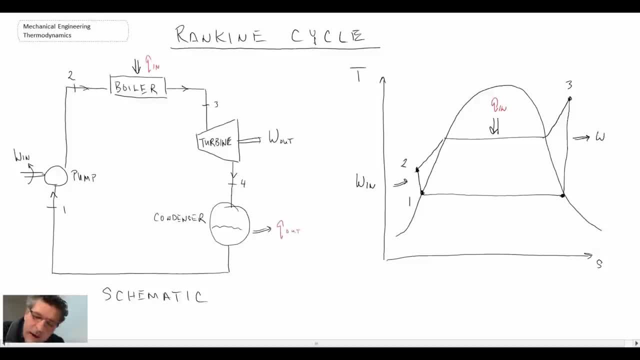 at state four, And then we're going to go into the turbine and we're going to drop down through the boiler And in the process of doing that we are producing work. And then, finally, from state four, returning to state one, we go into the condenser And in the condenser, 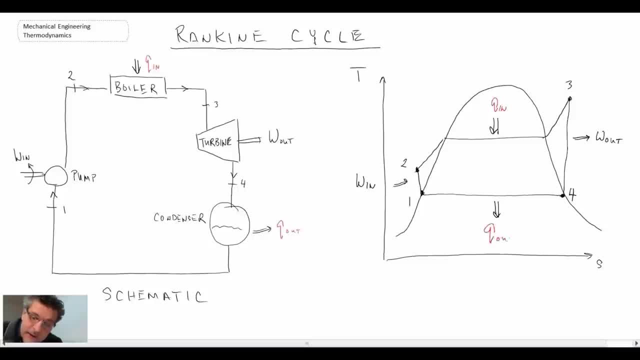 what we do is we are rejecting thermal energy to the environment, as all heat engines need to do. So that is the process diagram for the Rankin. So what we're now going to do is we're going to take a look and apply the first law to each of the individual components that are in the Rankine. 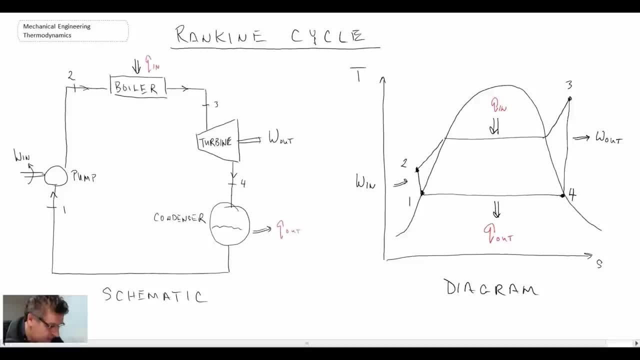 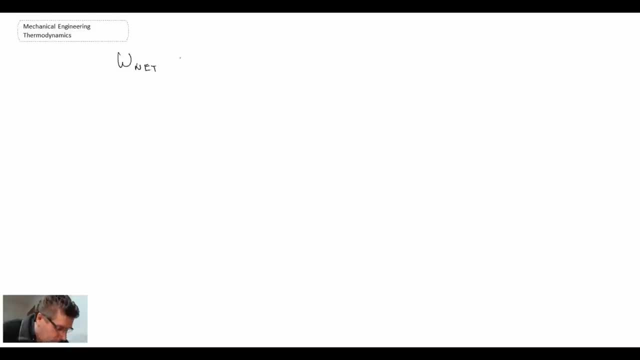 cycle. So let's begin by writing out an equation for the net work. We can say: the net work is going to be the work out minus the work in, and that can also be expressed in terms of the heat transfer: the heat in minus the heat out. So we're now going to apply: 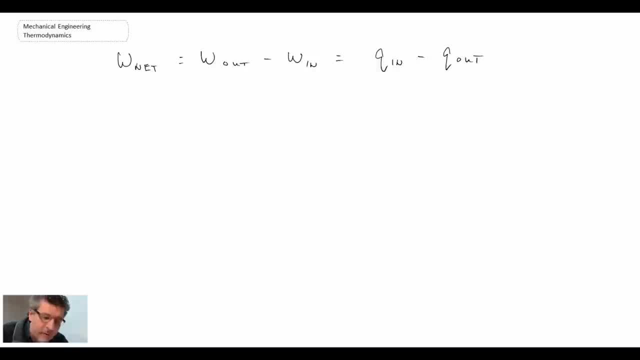 the first law to each of the components and we'll assume them to be steady flow components or steady flow devices and consequently, we'll use the steady flow version of the first law, So expressing or writing out the first law for a steady flow device. we have the following for our heat transfer: 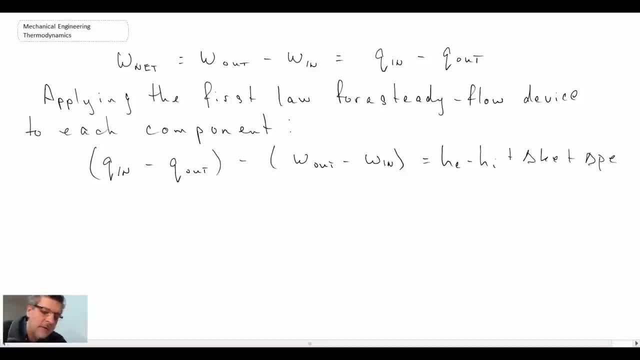 Now we're usually dealing with a device that's stuck to the ground, it's not moving and consequently we will take kinetic and potential energy and neglect those. So the first component that we will look at will be the pump, And in the pump, if you look back to 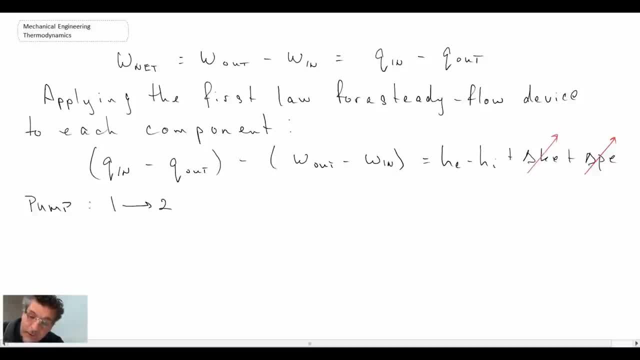 the process diagram and the schematic on the previous slide. in the pump we're going from state two to state two, So let's take a look at that Now. in the pump we can assume that there is no heat transfer, so Q will be zero And with that, when we come back to our first law, what we will have. 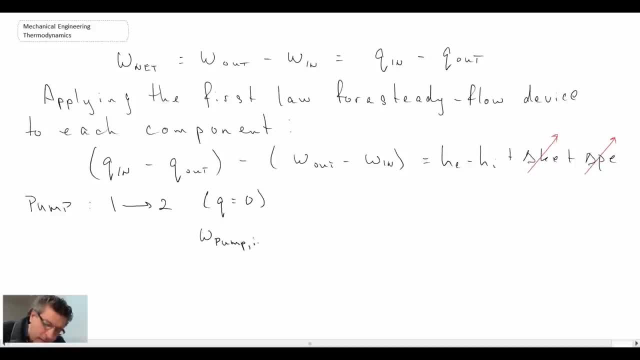 is the following for the pump: It's basically just the change in enthalpy. So we need a way to be able to express the change in enthalpy in the pump from the state two. So we're going to take a look at that. 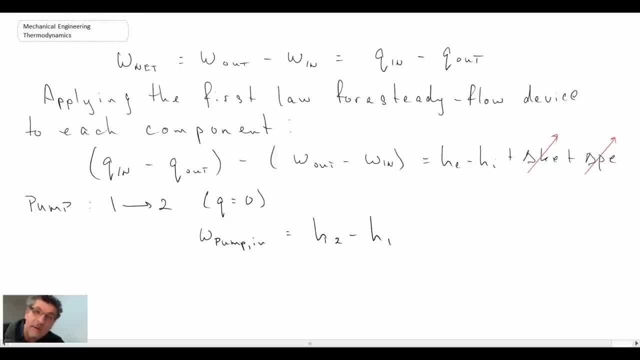 So we're going to take a look at that. So we're going to take a look at that And, in order to get that expression, what we'll be doing is we'll be using the steady flow work equation that we saw in an earlier lecture. 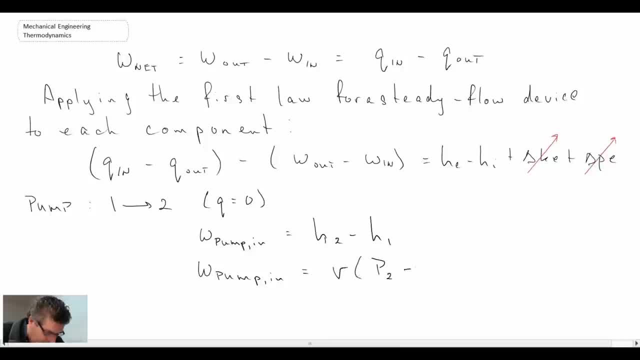 And, if you recall, this is the one that had the specific volume multiplied by the change in pressure of the fluid as it went through the device. Now, in coming up with this equation, what we're going to assume is that the enthalpy at state one 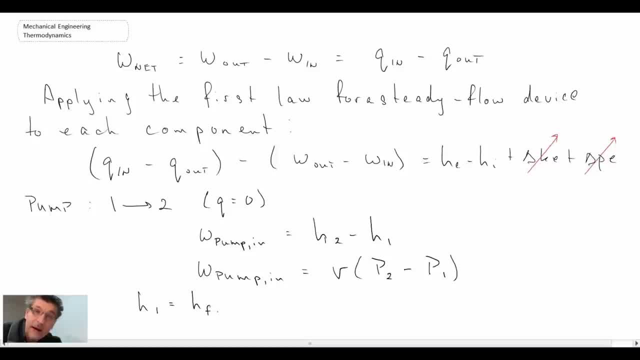 we will determine that by the enthalpy of a saturated liquid at pressure one which makes sense. We go into the steam table and we can get enthalpy there. But the question, how do we handle the specific volume? And the convention that we will use is: the specific volume will be the specific volume also at state one. 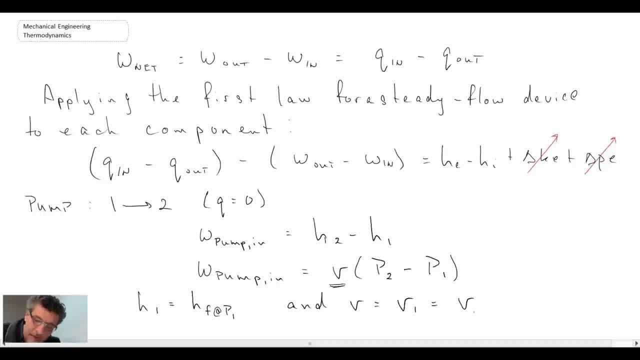 which would then be the specific volume for a saturated liquid at pressure one P1.. So that would be the pressure going into the pump, And you determine your specific volume there. You usually know the pressure differential And from that you can determine the work that you're putting into the pump. 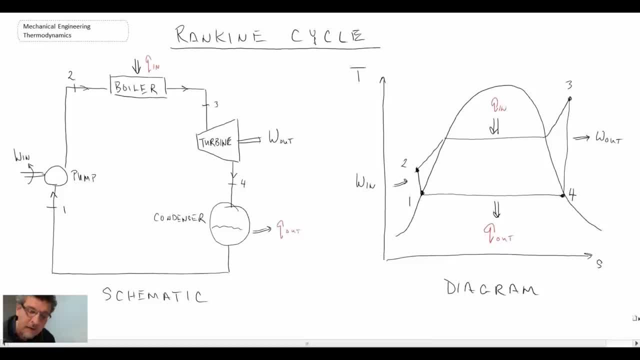 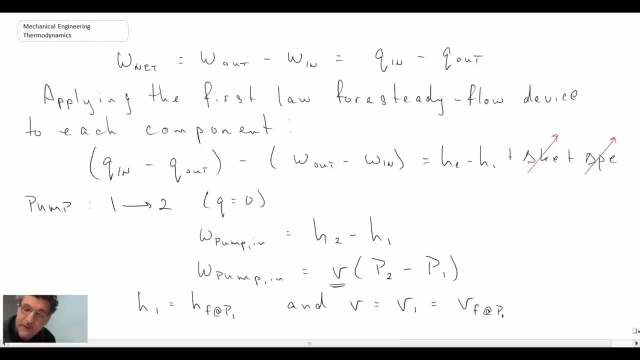 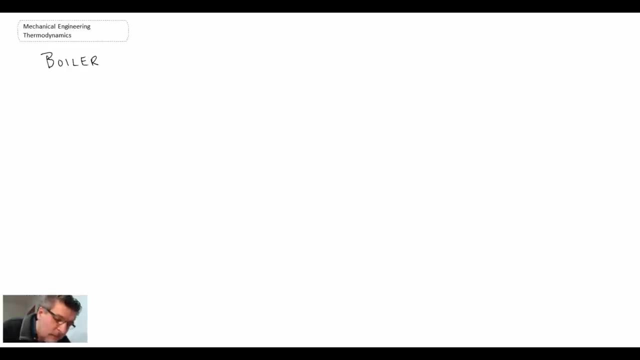 So let's move on to the next element that we have in our cycle, And that is the boiler. So let's apply the steady flow version of the first law to the boiler. So here we're going, from state two to three. Now, in the boiler, unlike the pump we said, there is no heat transfer. 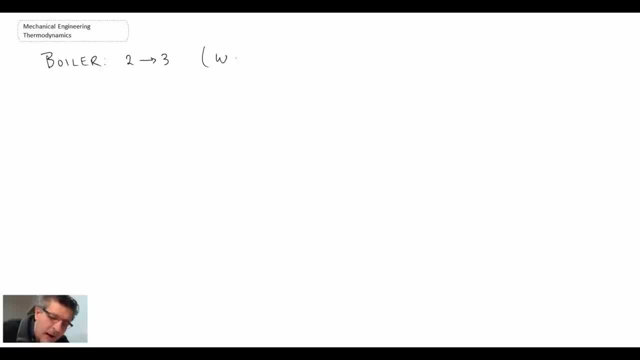 In the boiler there's a lot of heat transfer. That's what's making it work. However, there is no work in the boiler, So we can write: work is equal to zero. And then the steady flow version of the first law turns out to be the following: 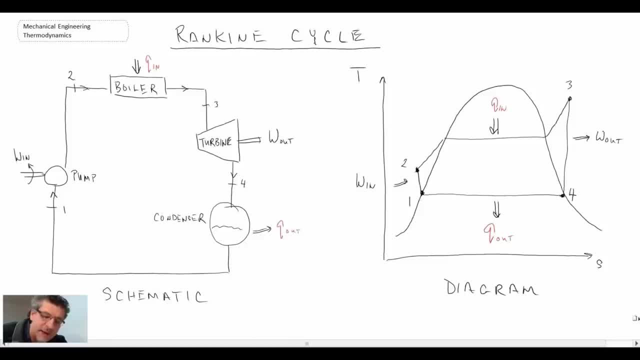 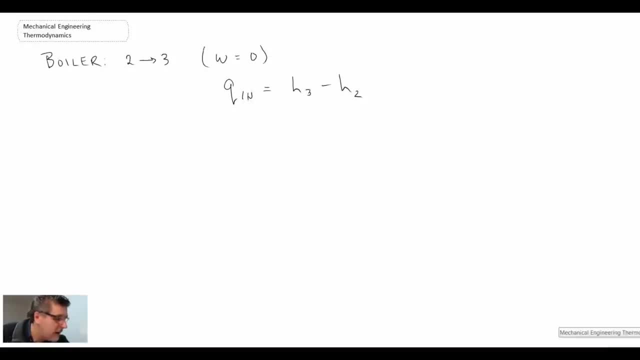 And so it's pretty simple. It's just the change in enthalpy that we have going across the boiler between state three and state two. Now the next item that we will look at is the turbine. Now, in the turbine, we're going from state three to state four. 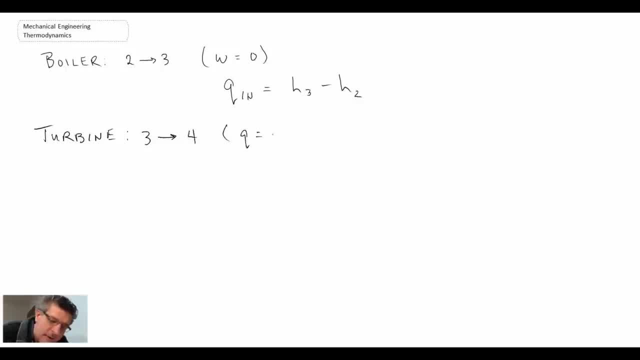 And in the turbine, just like in the pump, we're going to assume that there is no heat transfer And the only thing going on in the turbine is we're getting work out And the way that we will quantify that is going to be the change in enthalpy of the fluid going through the turbine. 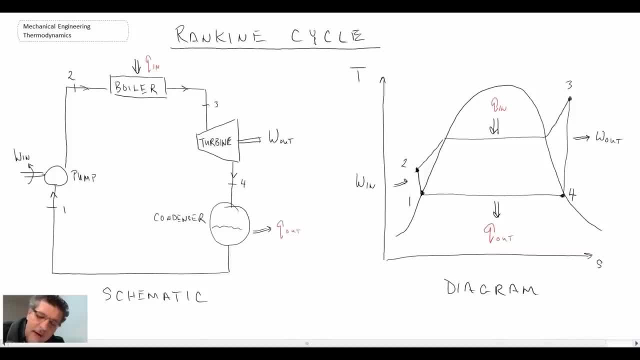 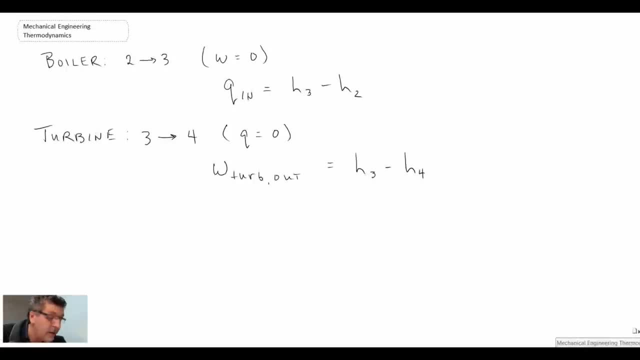 So, looking back at our TS diagram, it will be H3 minus H4. So that difference is how we can then determine the work in the turbine, And that will be pretty easy because we can get those enthalpy values out of the superheated steam tables. 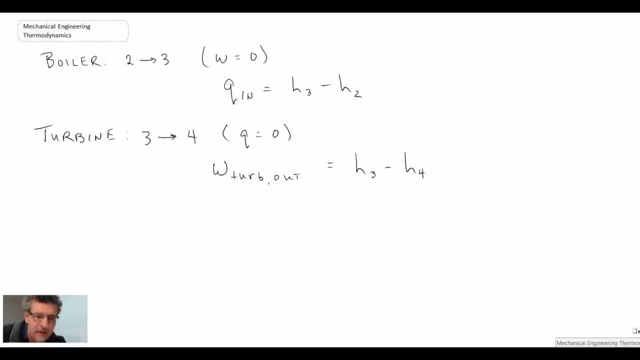 assuming we end right on the saturated liquid line. If we go into the two phase region then you have to look at the two phase characteristics there to get the enthalpy at state four. The final thing that we have is the condenser. 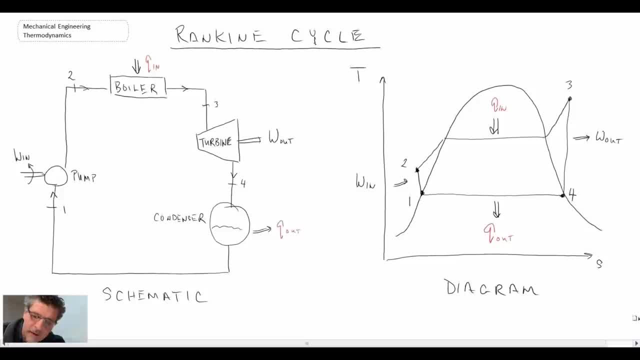 And for that we're going from state four to state one, going back here. So this is the operation of the condenser. It's basically heat rejection. We're going through a phase change. In an ideal world we go from saturated liquid. 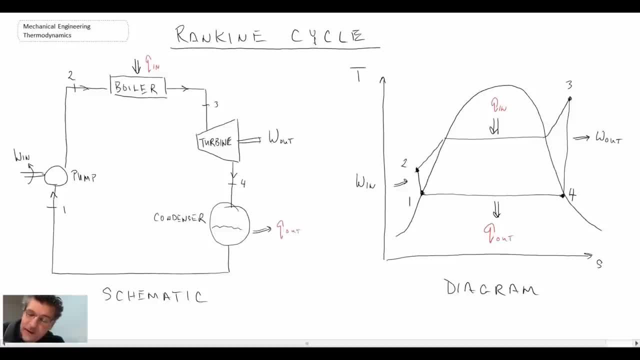 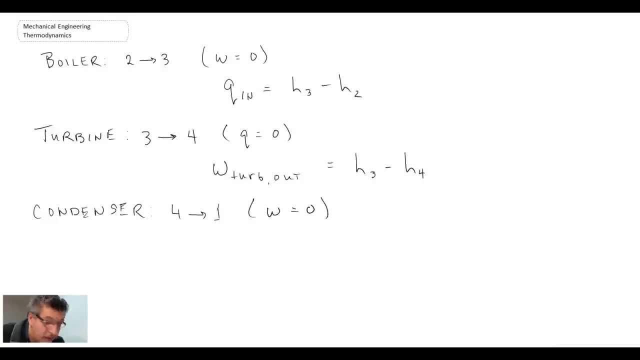 sorry, saturated vapor down to saturated liquid And consequently there is no work in the condenser. However, there is heat transfer. The heat transfer is leaving the system And that would be the enthalpy at four minus the enthalpy at one.